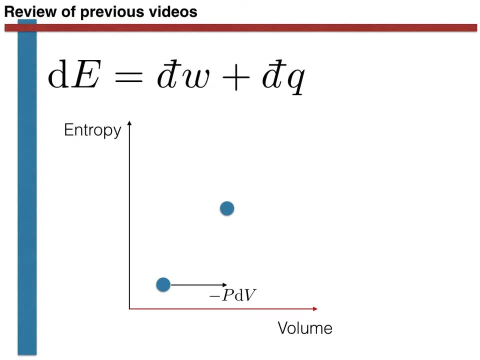 changes and the change in internal energy that occurs as we move parallel to the entropy axis, which we can calculate through the second law of thermodynamics. The final result is that dE equals TdS minus PeV. In these last few videos I want to focus on some of the 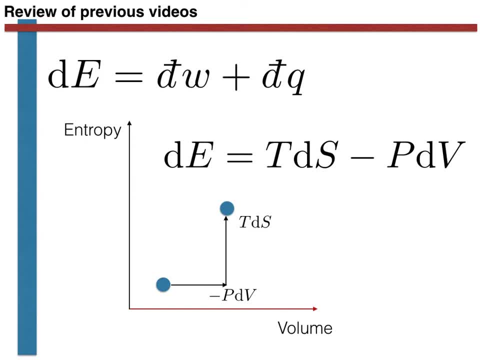 practicalities associated with using thermodynamics to solve thermal equations. This is because, if we apply these laws of thermodynamics and the determinations that occur within a system solve problems. In particular, I want to introduce a framework that will allow us to operate at constant temperature and constant pressure, rather than working at 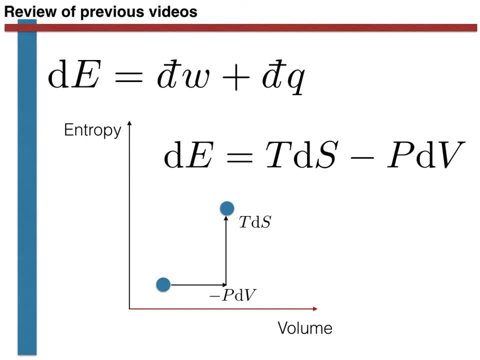 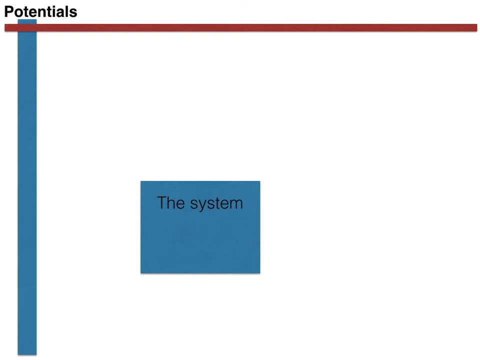 conditions where the entropy and volume are fixed. The notion of a thermodynamic potential is going to be critical to this process. We have seen potentials when we discuss Newton's third law. In that video I explained how we introduce potentials to describe the transfer of momentum between the system and the 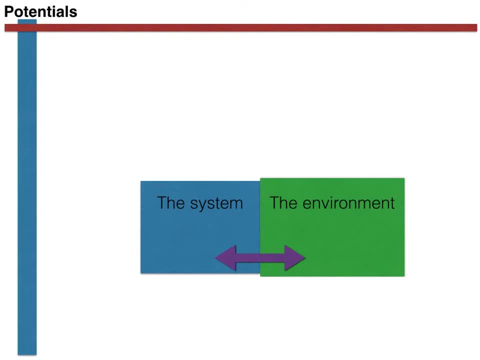 universe. If you remember, I explained how this makes our life much easier, as it allows us to model the coupling between the system and its surroundings without modeling every particle in the universe explicitly in our equations. In other words, we modeled the effect the universe has on the system in an averaged way. Our 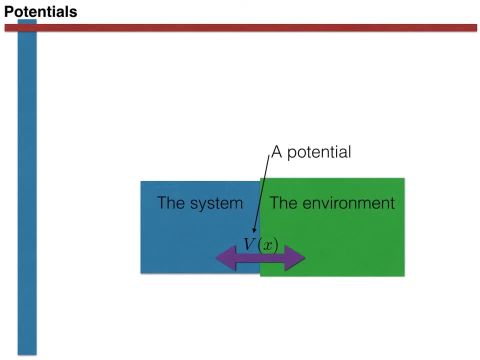 aim in this video will be to design a system based on the transfer of momentum between the system and the universe and thus introduce the notion of a thermodynamic potential, so that we can pull the same trick within the theory of thermodynamics. Before we get into that, let's just quickly review what we learnt about phase. 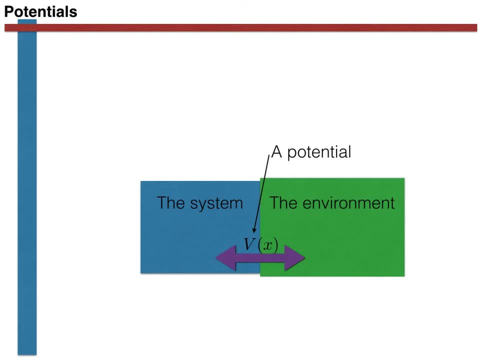 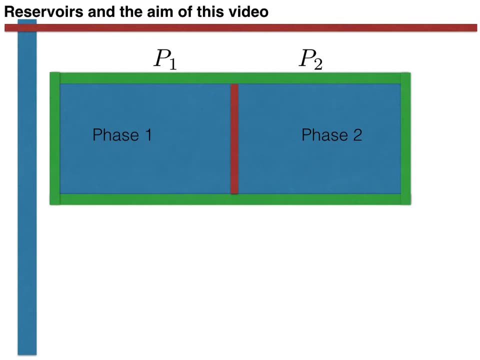 equilibrium and the way that the system interacts with its surroundings. We said that if we have two phases, as shown here, and if these two phases have different values for their pressures, or different values for any intensive quantity, for that matter, then they will exchange the conjugate extensive quantity in this. 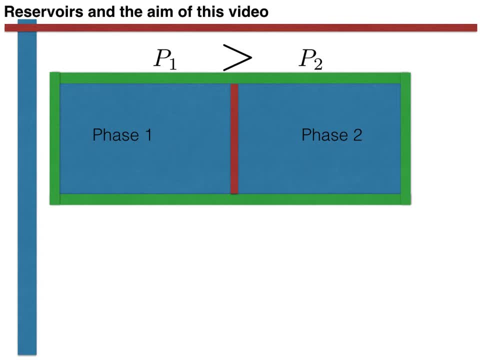 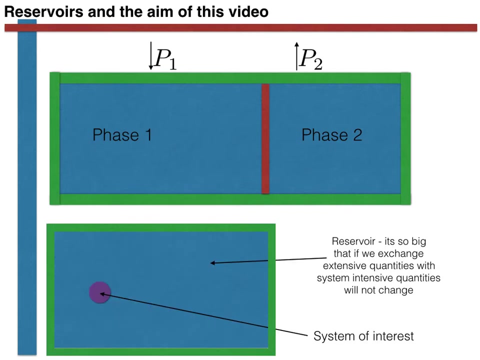 case, volume, until the pressures are equal. Thus, in the example shown here, the volume of phase one increases, thereby lowering its pressure, and the volume of phase two decreases, thereby increasing its pressure. Before introducing our notion of a thermodynamic potential, we need to introduce a reservoir. 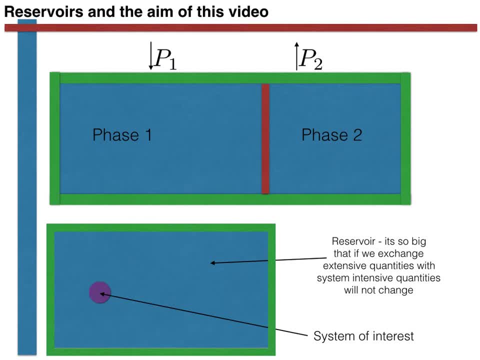 A system and a reservoir is a special kind of two-phase system in which one of the phases- the reservoir- is enormous. We can use a reservoir to model the interaction between our system and the rest of the universe. Furthermore, because the reservoir is huge, we can safely 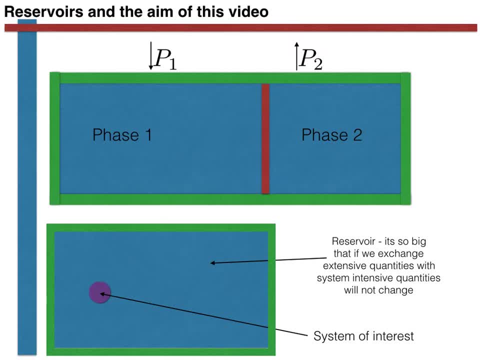 assume that when extensive quantities are exchanged between the system and the reservoir, the values of the intensive quantities in the reservoir do not change. As such. the values of the intensive quantity in the whole system do not change as heat or work is exchanged between the system and the reservoir. 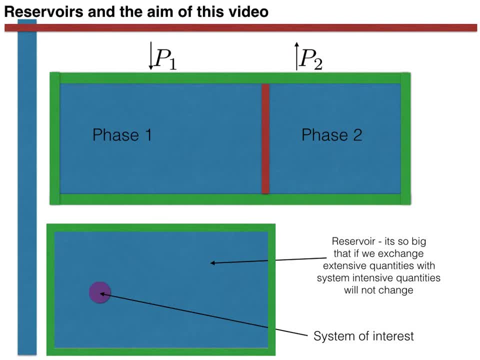 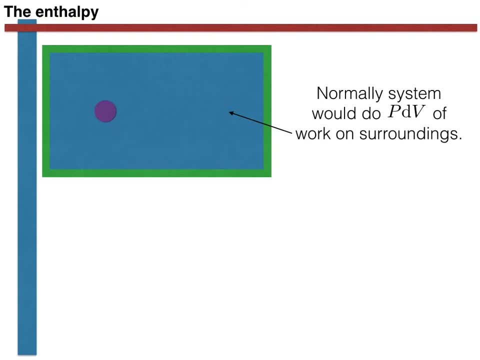 Allow me to explain what that means with an example. Suppose the purple phase. the system expands slightly. here Work will be done by the system on the reservoir. We know that the amount of work done on the system will be equal to minus PdV- Now normally an equal. 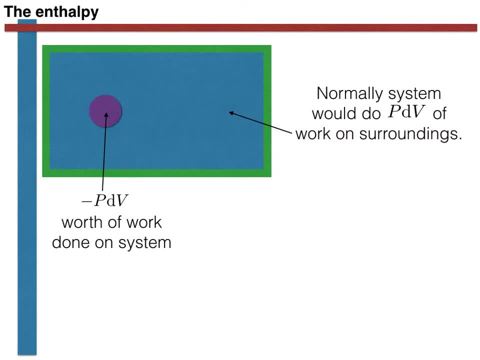 and opposite amount of work would be done on the environment In order to ensure that the total energy of the two phases is conserved. PdV's worth of work would thus be done on the reservoir. The volume of the reservoir would thus change. Herein lies the problem, though. 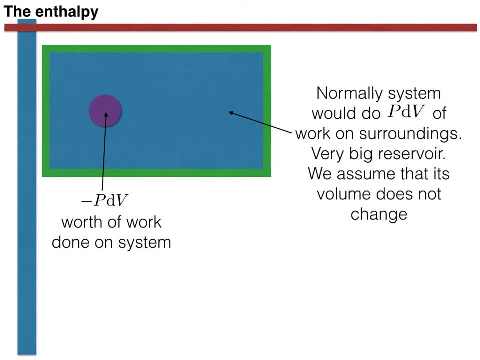 The reservoir is large. In fact, for all intents and purposes, we are going to assume that its volume is infinite. As the volume is infinite, it cannot change. Adding infinite anything to infinity gives us infinity again. We are thus left with a problem: The extra work. 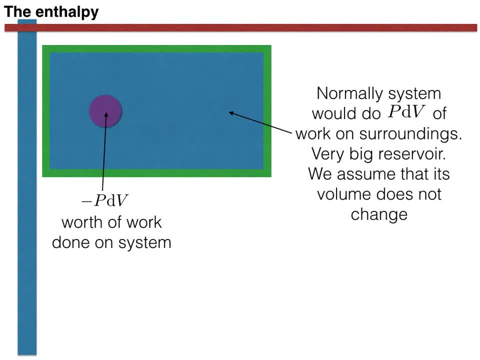 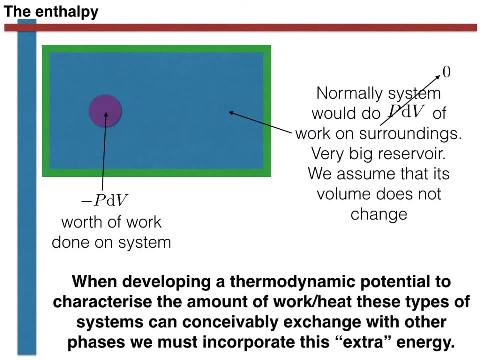 that would normally be done on the universe is lost because the volume of the reservoir does not change. We thus need to develop a thermodynamic potential that deals with this extra energy. We have to characterise the amount of work that the reservoir would do, as only then can we ensure that energy is conserved throughout our entire two phase. 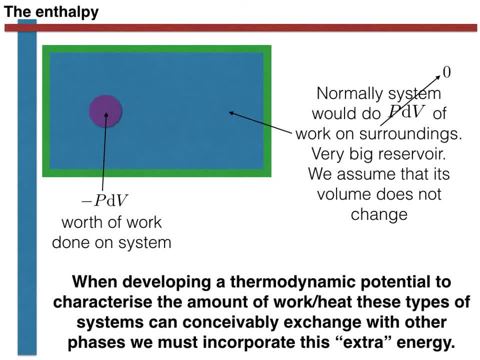 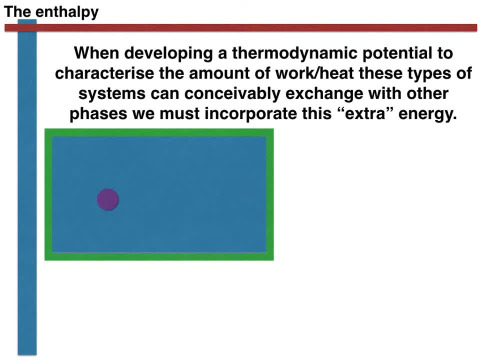 system. To do this, we proceed as follows: Instead of just keeping track of the energy of the system, we keep track of the change in energy plus the change in PdV. The second term here is the amount of work the reservoir does when either the pressure of the system, 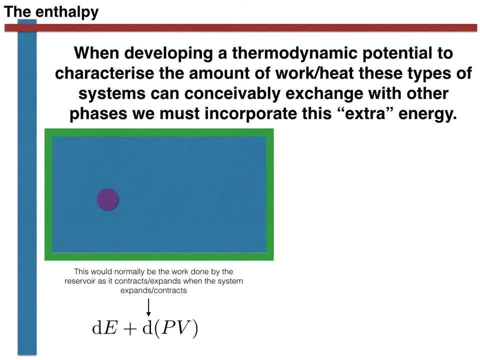 or the volume of the system changes. Remember that when the volume of the system changes, the amount of work done on it is equal to minus PdV. In other words, when the system expands, work is done on the universe. The sign of this new dPV quantity is thus positive, because we are using it to keep track. 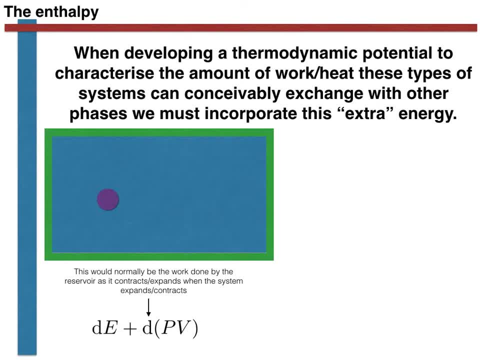 of the changes that take place in the reservoir. These have the opposite sign to the changes in work that take place in the system. We now proceed as follows. We can use the product rule to write dPV as PdV plus VdP. 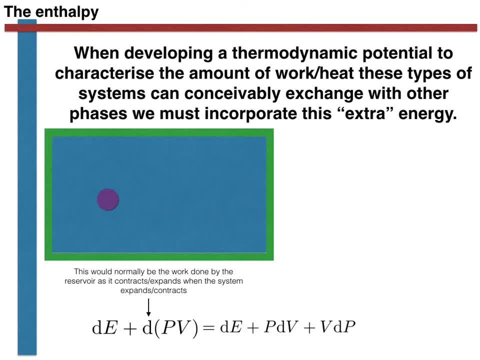 We then recall that dE equals TdS minus PdV. The minus PdV and the plus PdV terms then cancel and we are thus left with TdS plus VdP. This sum is the change in a new thermodynamic. 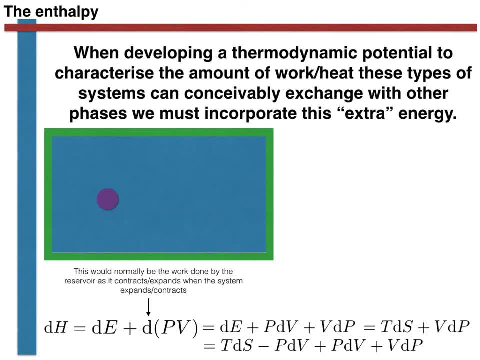 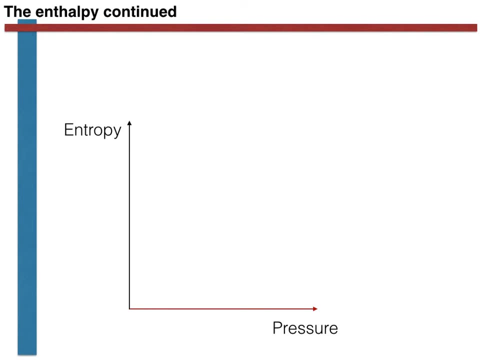 potential we call PdV. The enthalpy is given the symbol H and thus an infinitesimal change in this quantity can be written as dH. Enthalpy, like internal energy, entropy, volume and all the other extensive thermodynamic variables, is a function of state. As such, the change in enthalpy on moving between two 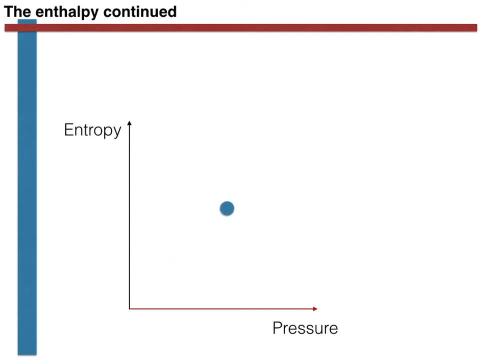 states does not depend on the path taken. We can thus always calculate the change in enthalpy by considering a root, when we move between our two states, at first along a path parallel to the pressure axis, and by then moving along a path parallel to the entropy axis. 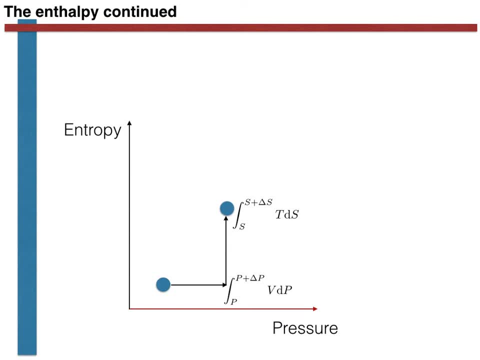 To calculate the changes in enthalpy along these paths we perform the definite intervals shown here. This is just another way of analyzing the change in enthalpy. so if we look at the expression understanding, the expression we derived on the previous slide, that relates an infinitesimal. 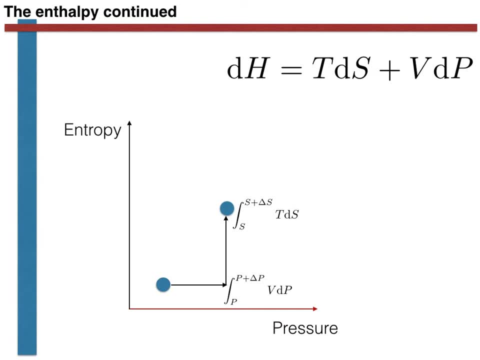 change in the enthalpy to infinitesimal changes in pressure and entropy, Remembering from the theory of partial differential equations that we can always write such infinitesimals, as shown here and equating terms, allows us to connect the temperature with the partial derivative of the enthalpy with respect to entropy at constant pressure. 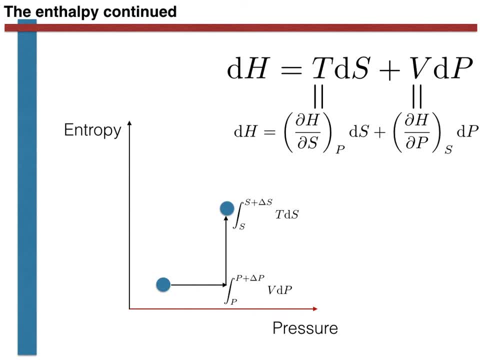 and the volume with the partial derivative of the enthalpy with respect to pressure at constant entropy. An alternative way of thinking about these derivatives is to remember that differentiation is the reverse of integration. If I thus take the integral, that gives me the change in enthalpy that I would observe if I change the pressure whilst holding. 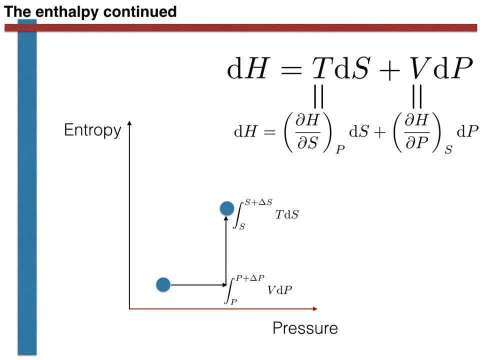 the entropy fixed and differentiate this with respect to the pressure, I get that the derivative of the enthalpy is the partial derivative of the enthalpy with respect to the pressure. at constant pressure is equal to the volume. Similarly, if I take the equation that gives me the change, 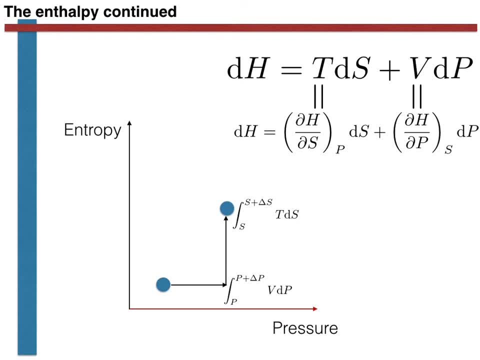 in enthalpy that I would observe. if I change the entropy whilst holding the pressure fixed and differentiate this with respect to the entropy, I get that the derivative of the enthalpy with respect to the entropy at constant pressure is equal to the temperature. 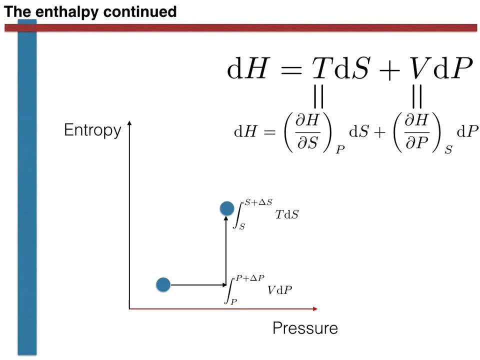 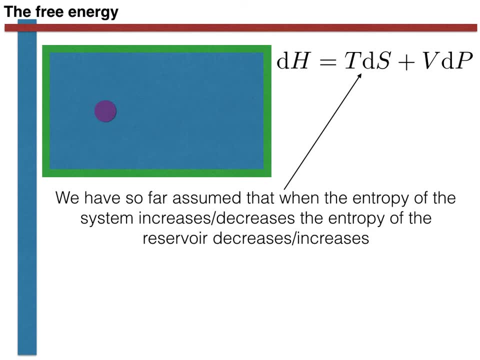 Let's now move on to a second kind of thermodynamic potential. We have thus far assumed that when the entropy of the system increases, the entropy of the reservoir decreases. In other words, we have assumed that entropy is transferred from the system to the reservoir so that any 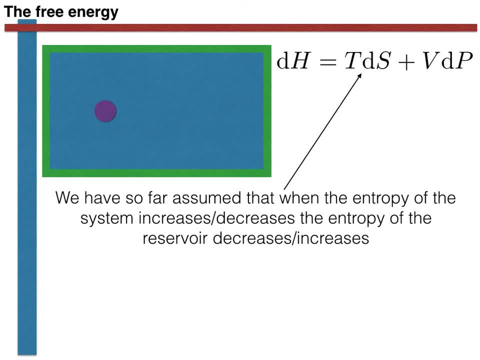 decrease in the entropy of the system is counterbalanced by an increase in the entropy. What we are now going to do is look at a reservoir whose volume decreases when the system expands. When this reservoir exchanges entropy with the system, however, its temperature will not change. 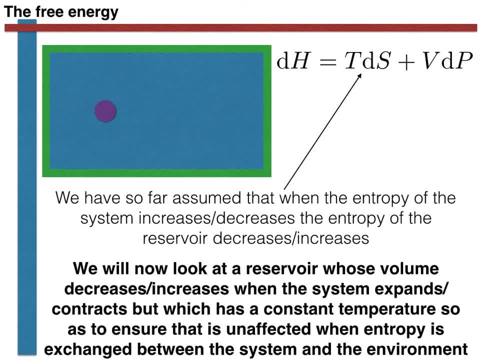 Much as we did with the volume in introducing the entropy. we will thus assume that the entropy of the reservoir is, to all intents and purposes, infinite, And this is the reason that exchanging entropy with it makes no difference to the temperature. Adding or subtracting any finite number from infinity gives infinity. 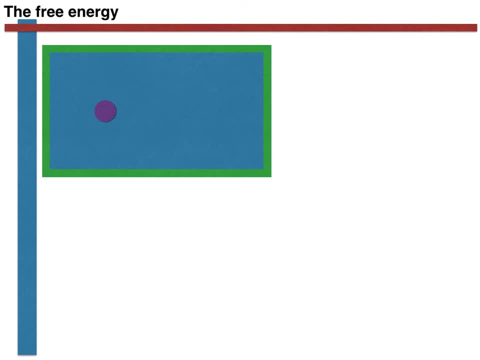 Let's just quickly summarise this all diagrammatically. Here is our purple dot representing the Syrris system, surrounded by the very large blue reservoir. The entire system is then surrounded by a set of walls that are the same size as the entire reservoir. 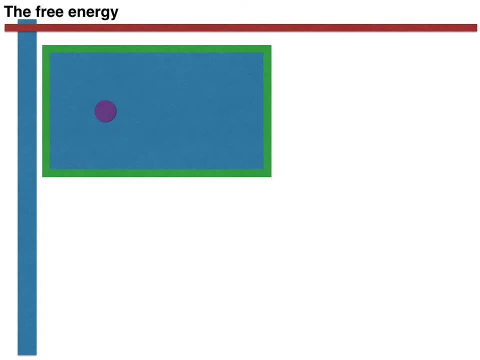 The entire system is then surrounded by a set of walls that are the same size as the entire reservoir. The entire structure makes sure that the whole two-phase system does not exchange matter, heat or work with its surroundings. The total energy of the system and the environment are thus constant. 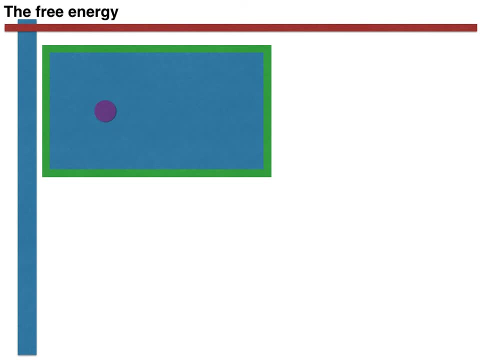 Let's now suppose that something happens within the system so that heat is exchanged with the reservoir. As we have learnt, if Tds worth of heat is transferred from the environment to the system, then the internal energy of the system will increase by TDS. 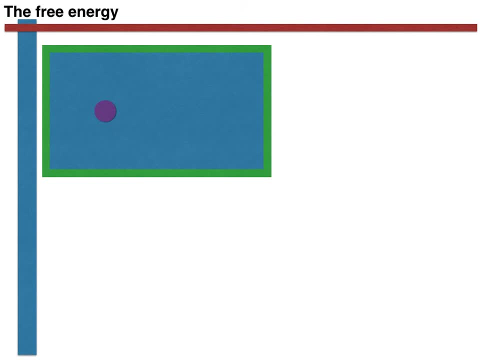 while the internal energy of the environment will decrease by TDS. This all assumes that the volume of the system in the reservoir remains constant throughout the process, however. Remember, though, that we are assuming that the system is very large and that, as such, the entropy of it does not change. 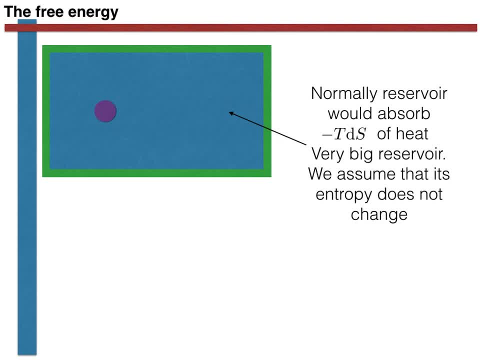 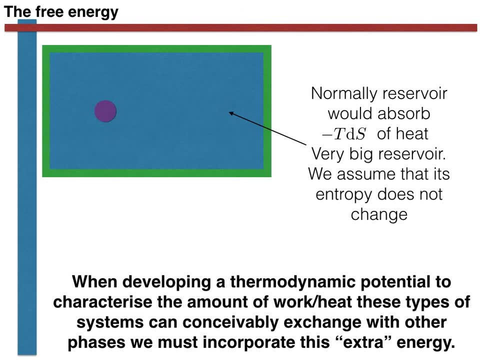 when this piddling amount of entropy is transferred into it. We must therefore develop a thermodynamic potential that is able to keep track of the total amount of heat and work done within the system and that also keeps track of the amount of heat. 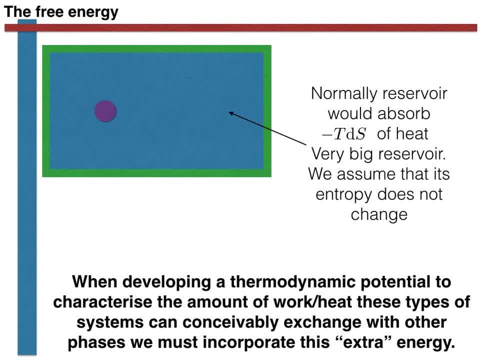 that would normally have been absorbed by the reservoir. In other words, in order to ensure that energy is conserved throughout the universe of our system and reservoir, we must keep track of this extra energy, the energy that would normally be absorbed by the reservoir. 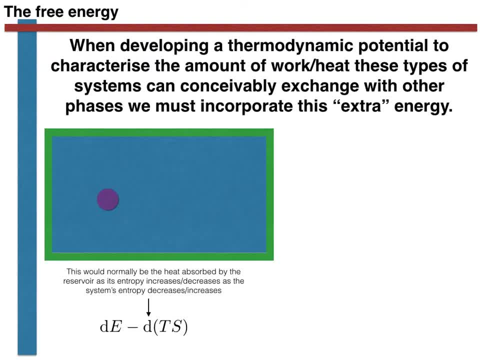 We must therefore consider the infinitesimal shown at the bottom of this slide, which consists of DE- the change in the internal energy of the system, and DTS- the heat that would normally be absorbed by the reservoir as the entropy of the system increases or decreases. 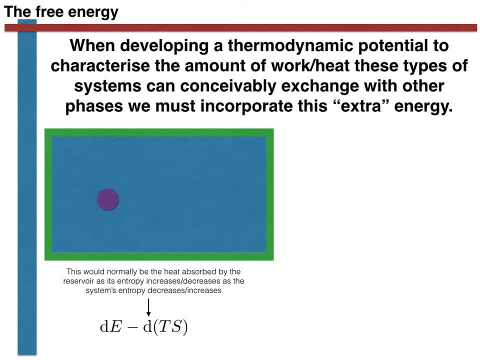 Expanding out the factor of DTS using the product rule, we arrive at the following: We then remember that we can write the DE as TDS minus PV. The factors of plus TDS and minus TDS then cancel and we arrive at the following: infinitesimal. 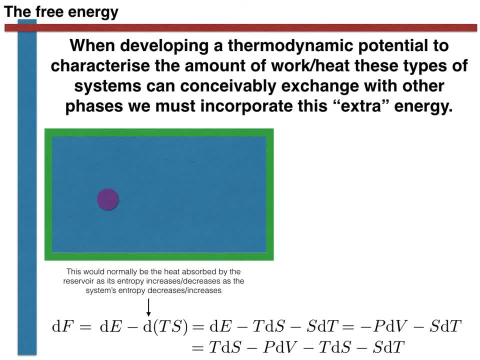 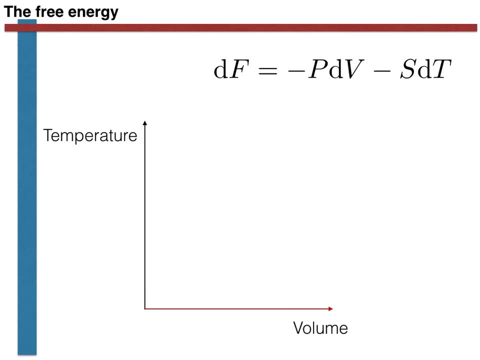 which is the amount. a new thermodynamic potential called the Helmholtz free energy F, changes when the volume or temperature of the system is changed. Once again, this new thermodynamic potential, the Helmholtz free energy, like internal energy entropy volume, 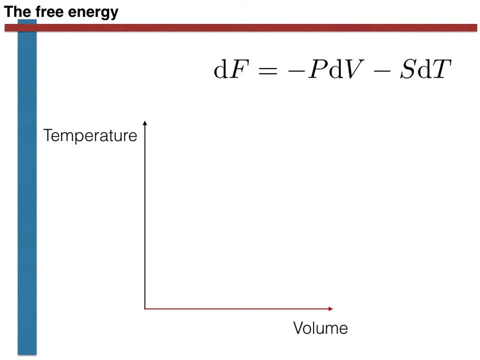 and all the other extensive thermodynamic variables is a function of state. As such, the change in Helmholtz free energy that occurs on moving between two states does not depend on the path taken. We can thus always calculate the change in free energy. 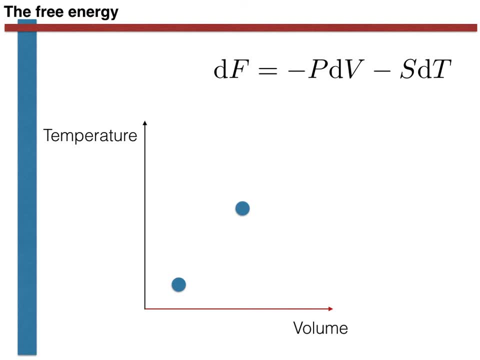 by considering a route where we move between our two states at first along a path parallel, parallel to the volume axis, and then by moving along a path parallel to the temperature axis, To calculate the change in free energy along these paths, we perform the definite integral shown here. 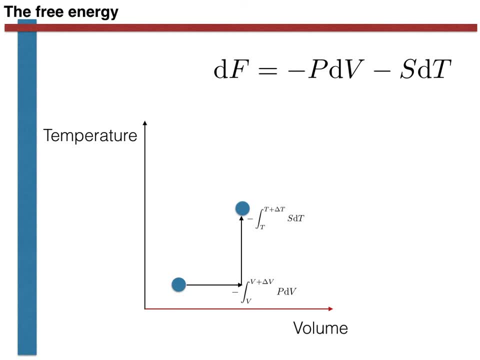 This is just another way of understanding the expression that we derived on the previous slide that related an infinitesimal change in the Helmholtz free energy to infinitesimal changes in the volume and temperature, Remembering from the theory of partial differential equations that we can always. 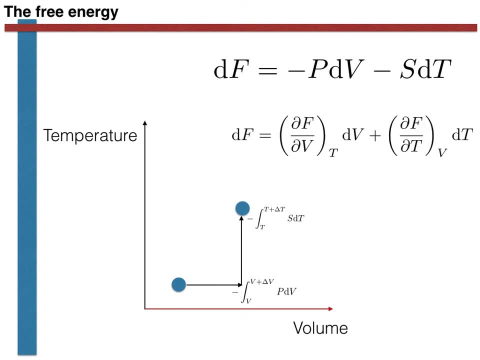 always write such infinitesimals as shown here, and equating terms allows us to connect the entropy with the partial derivative of the free energy with respect to temperature at constant volume, and the volume and the pressure as the partial derivative of the free energy with respect to the volume at constant temperature. 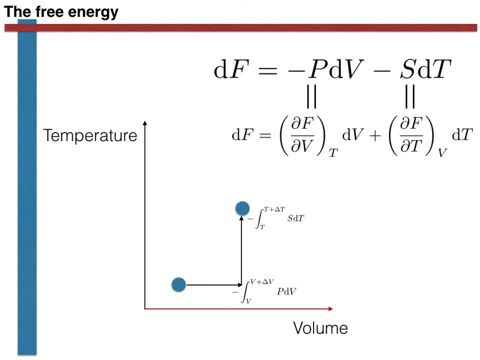 Much as with the enthalpy case, we can understand where these equations come from by considering the fundamental theory: Integration is the reverse of differentiation. Hopefully this has given you a flavour of how infinitesimals can be defined by using the properties of reservoirs.